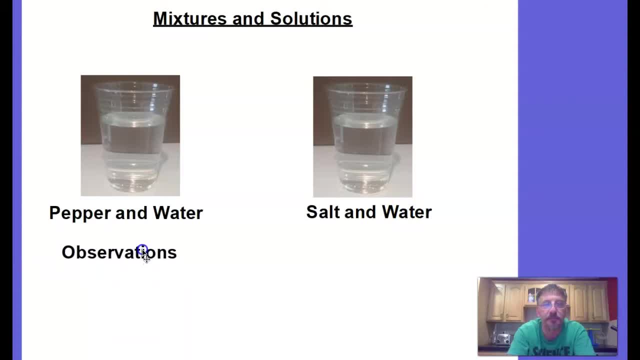 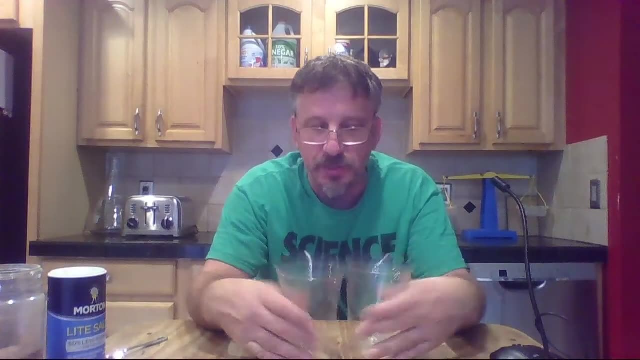 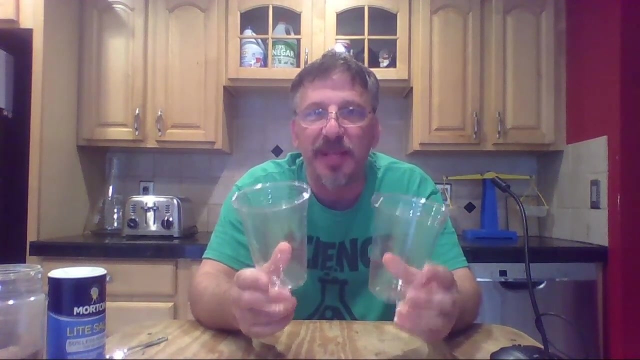 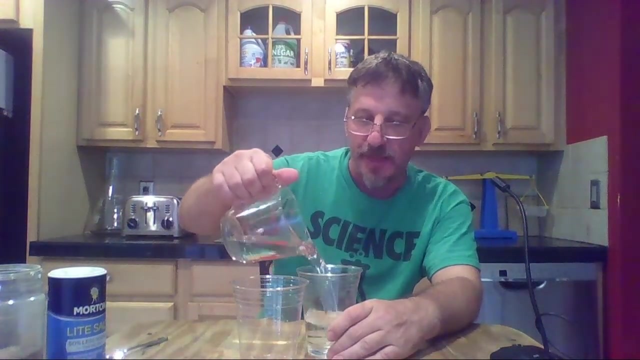 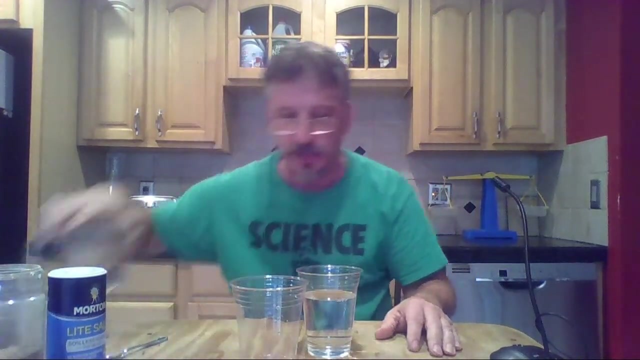 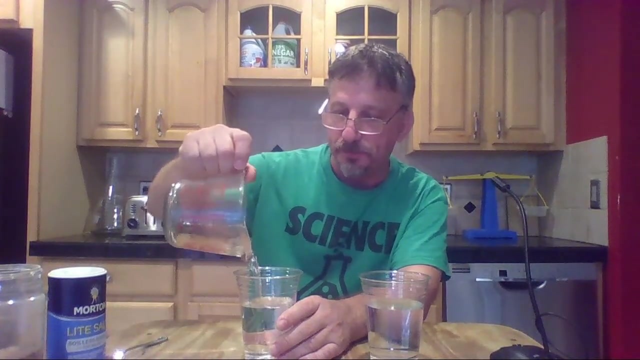 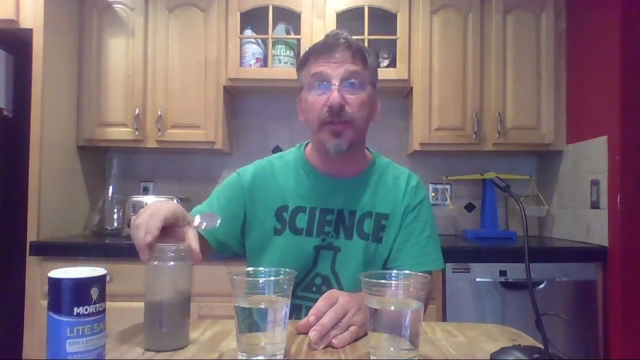 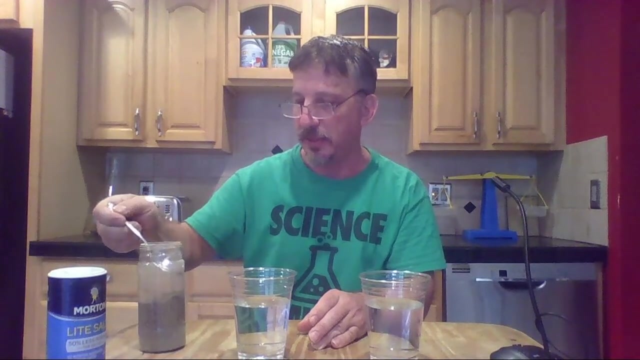 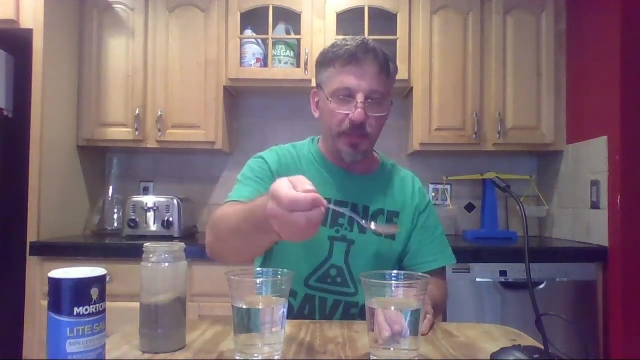 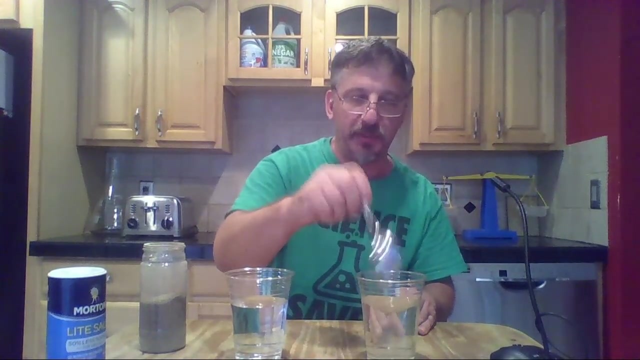 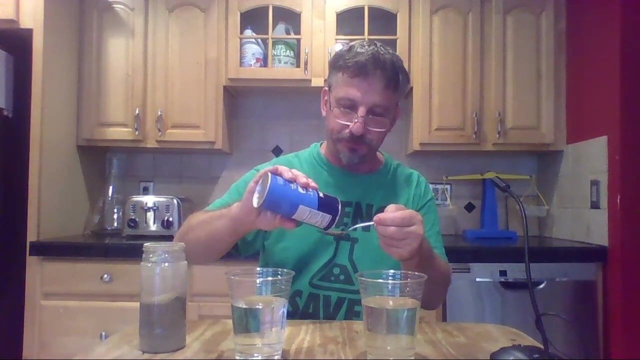 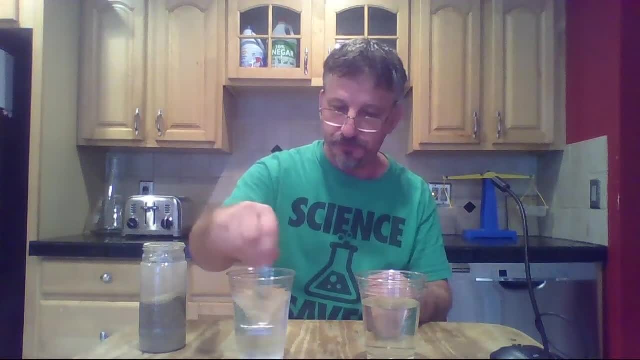 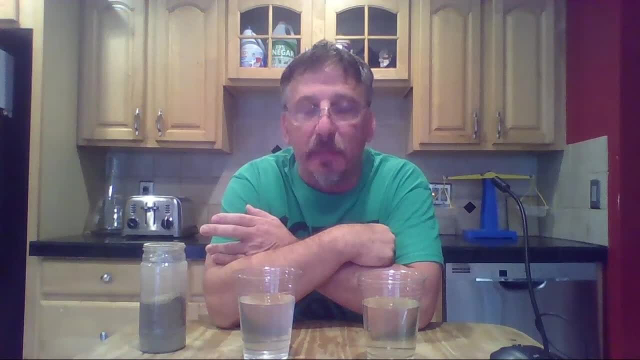 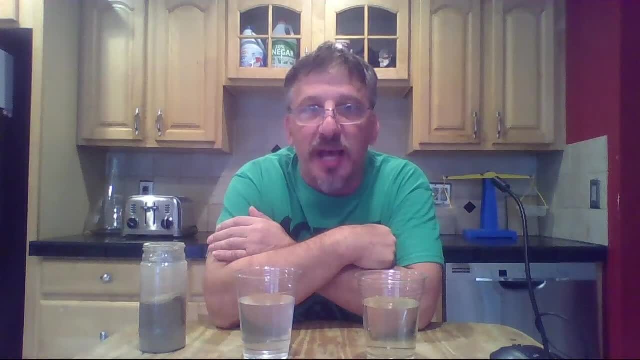 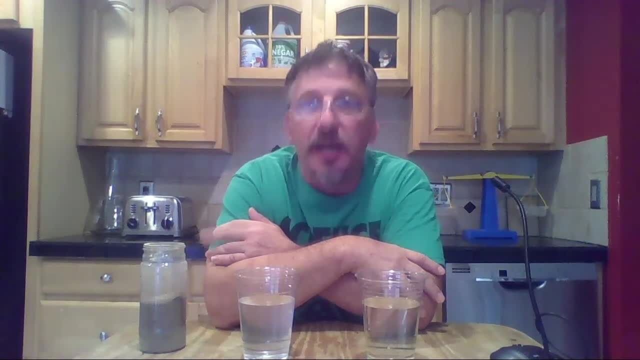 You can talk about that right now when you put it in your notes. Another thing I'd like to do is I'd like to talk about the texture of it. It's fine means it's kind of fine and smooth. A word like coarse means it's a little rough. 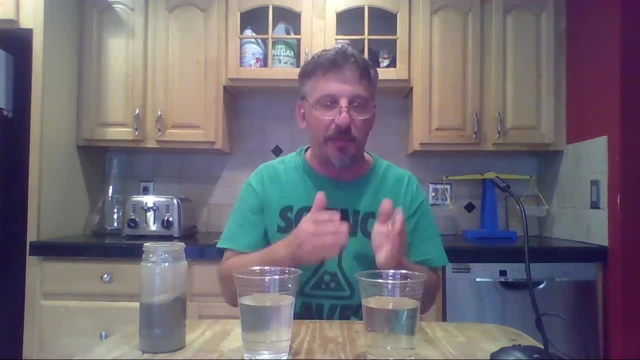 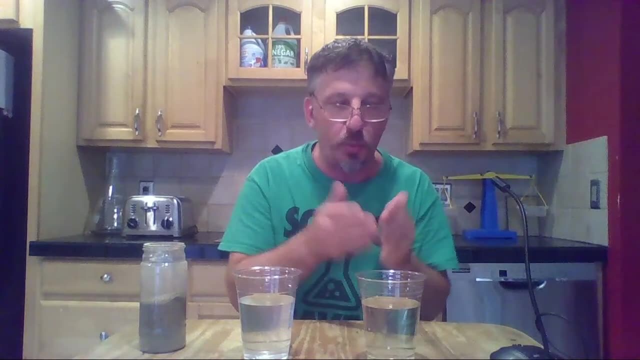 So those are other things you can talk about. So anything you can say about each one. Now we drew both cups, So under the pepper and water cup, write down everything you observe. What do you see? What's happening? Same with the salt and water. 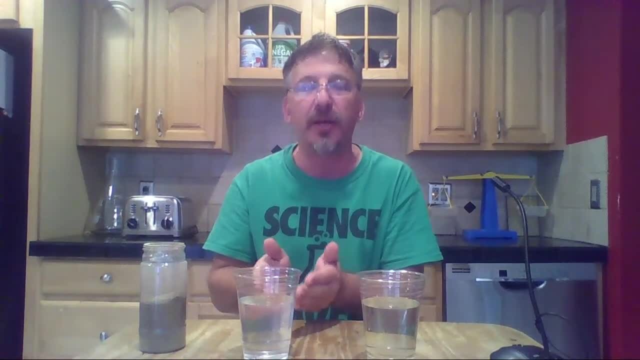 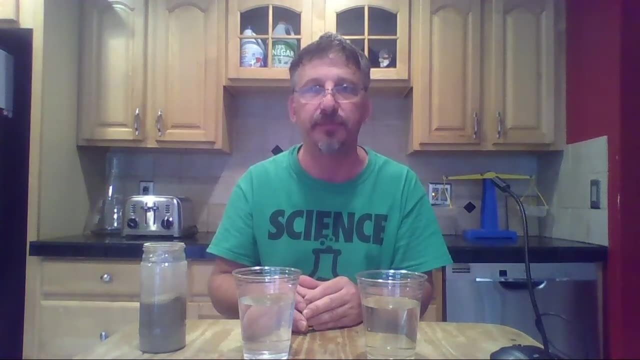 What do you see? What's happening? So take a few moments, go ahead and write all your observations, Be detailed, be specific, and we'll talk about it in a moment. Pause the video, All right. so the first thing I want to do is I want to fill in my diagram here. 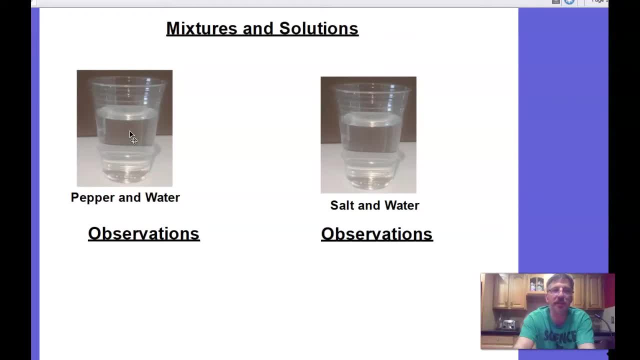 So it's different to be in a picture and a diagram is a picture is just a picture and a diagram has labels. So I told you before: we have three hundred twenty five milliliters of water. Now if you have a different amount of water, a different volume of water, then you should label your volume to what yours is. 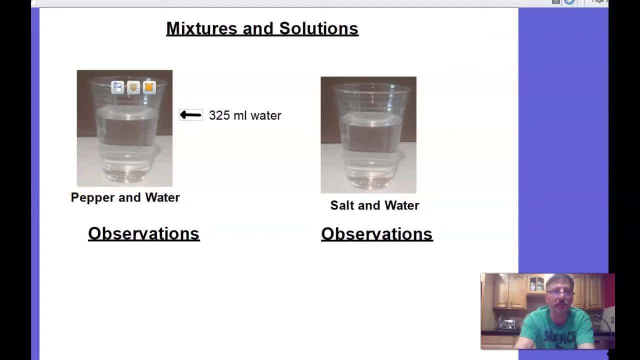 So I'm running three hundred twenty five for both of them And of course, you want to label it with ml for milliliters. So three hundred twenty five milliliters for both And you know I'm gonna go ahead and label it. 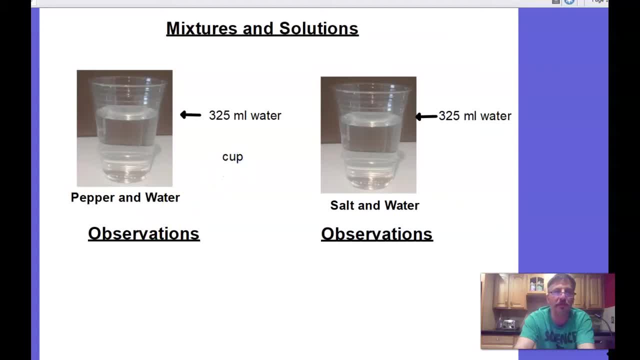 I'm gonna label it a cup too. I know, we know it's a cup, but we're gonna label it a cup. Now, what you're gonna want to do is you, wherever you have pepper, you're gonna want to, at least you want to put a little black dots with your pencil, or your pen or your mark, or whatever. 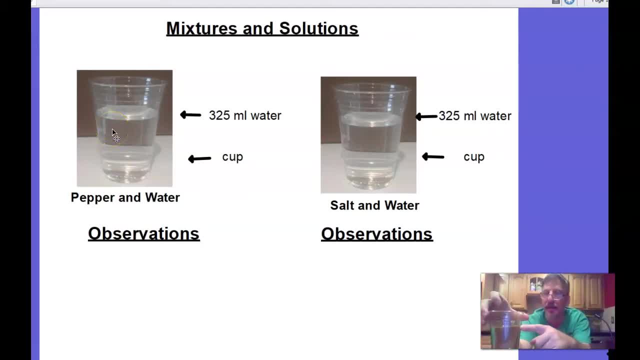 I have. I have it both on the top and the bottom. I have pepper that's floating on the top, I have some in the middle- It's sinking- and I have some along the bottom. So I would want to put a bunch of dots and just kind of. 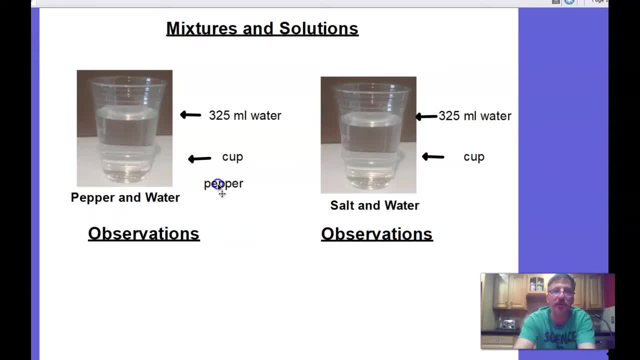 label it pepper and, you know, point to a few of them. You're obviously not going to point to every single one of them, But you want to point to a few of the peppers that you see. You draw a couple arrows here and there and whatnot. 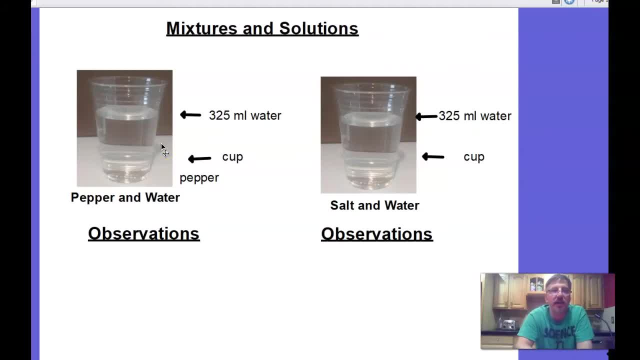 Then you want to be specific about your observations. Let's let's write some observations. I have very fine particles of pepper, So fine. Fine means small and smooth, So fine is something very small and smooth. I noticed, I observe, that some of my pepper floats and some of my pepper sinks 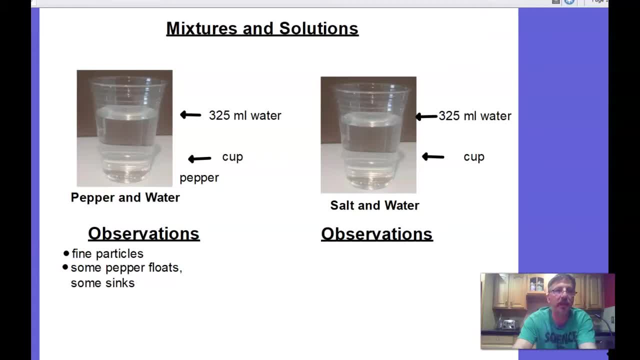 So I'm writing that Mine turned a little brownish So I put my water turned brownish And that's all I have. If you have more than that, the more you have the better. If you don't have some of the things I have, go ahead and write it. If you have more, well. 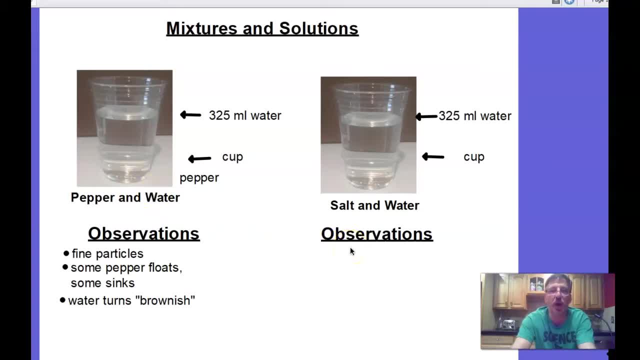 Well, that's great. Now I'm going to do my observations of salt and water. Well, I had fine particles to begin with, but I noticed that the salt disappeared. And it really didn't disappear, It dissolved. So I put salt dissolved. 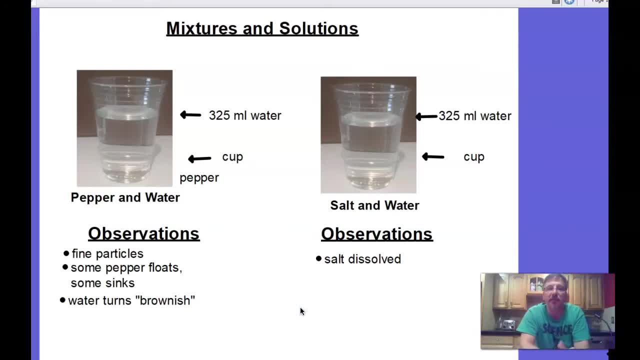 And the water is clear. You might want to write that, But that's what I have for my observations. So I hope yours is something like that And we're going to keep writing notes. We're going to talk more about which one's a mixture and which one's a solution. 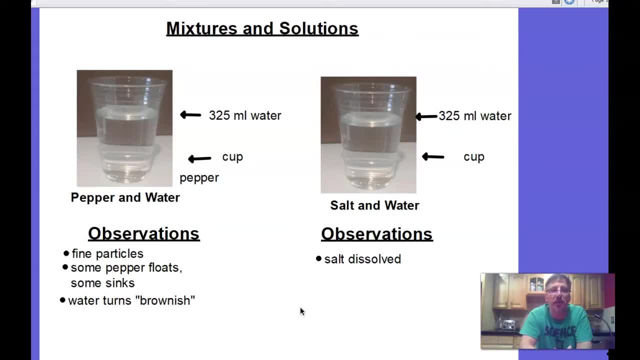 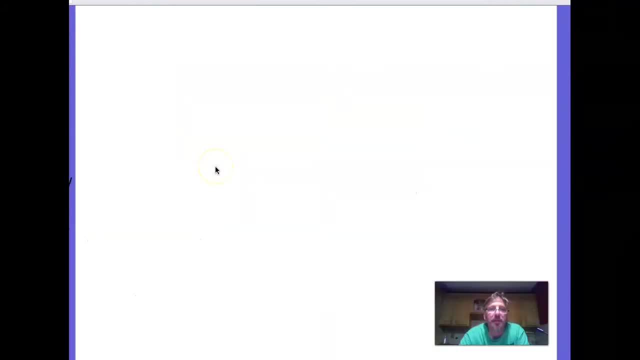 We're going to write some definitions and whatnot, So let's just keep going with the journal writing. Get all this copy, Pause the video And we'll get up to date here. All right, Skip a line And we're going to write some definitions. 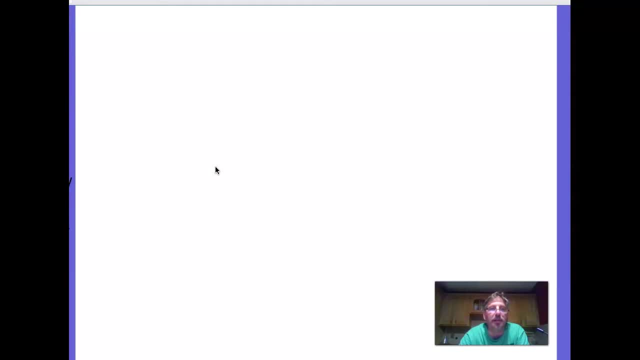 And eventually we're going to go back to the pictures, the black pepper and water and the salt and water, and decide which one's a mixture and which one's a solution. So skip a line And here we'll write a definition of mixture. 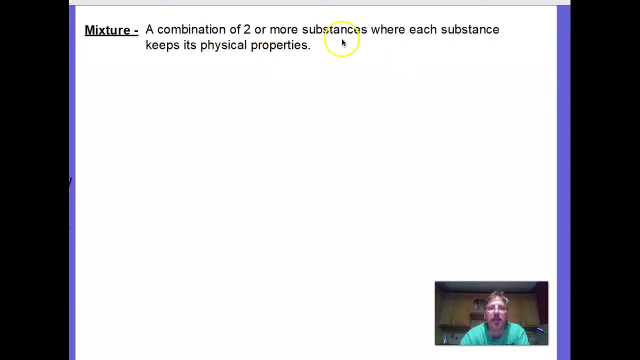 And a mixture is a combination. A mixture is a combination of two or more substances where each substance keeps its own physical properties. So go ahead and write that And then skip a line, and we'll write the definition of solution. And a solution is a type of mixture where one substance dissolves in the other substance. 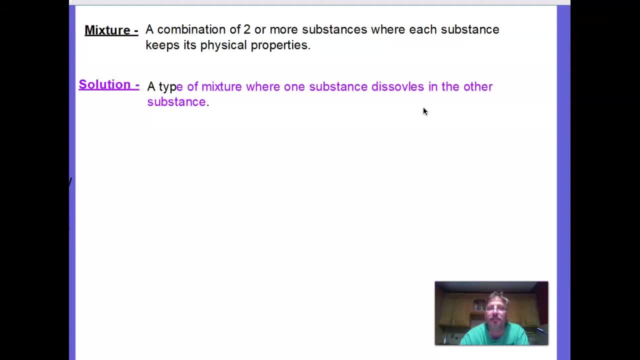 I bet a lot of you already know which one's which, don't you? All right, We're going to be making a list of characteristics of both mixtures and solutions, So you're going to need about a half a page. So if you are running out of room, go on to the next page and we'll make our list there. 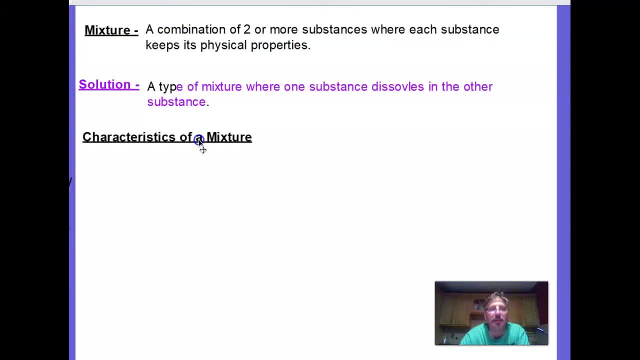 All right. So on the left side we're going to write the characteristics of a mixture, And on the right side we're going to write the characteristics of a solution. So we're going to make a bulleted list here, All right? 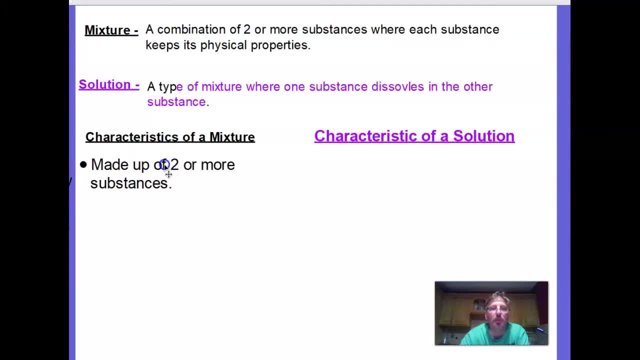 So if it's a mixture, it's made up of two or more substances. Well, both of them were that, weren't they? One was black pepper and water and one was salt and water. So they're both made up of two or more substances. 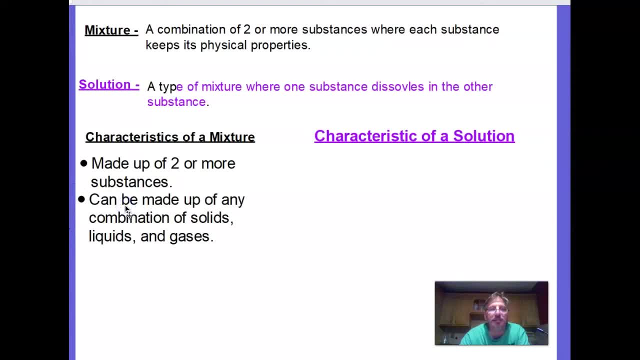 Secondly, can be made up of any combination of solids, liquids and gases. So what was the black pepper and water? What kind of combination was that? Well, the black pepper was a solid and the water was a liquid, So it was made a combination of a solid and a liquid. 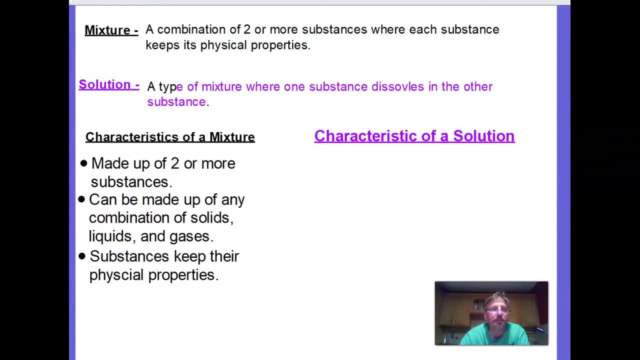 Substances keep their own physical properties. Each substance can be seen individually And often, but not always, can be separated. You could take each ingredient out. You could take each substance out. So why don't you go ahead and catch up with this list? 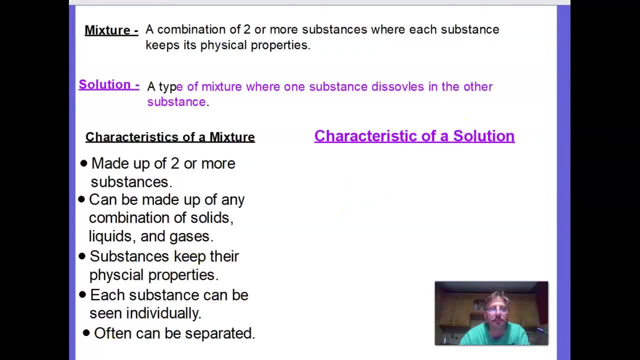 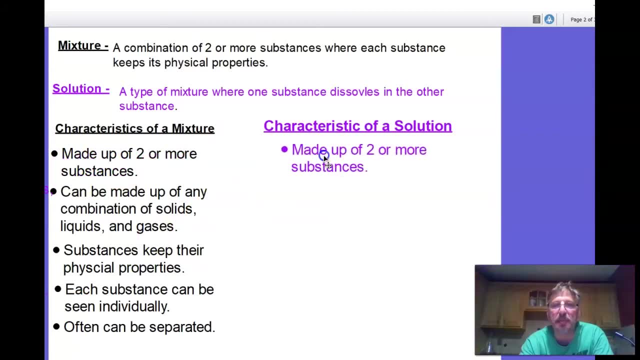 And then we'll go ahead and write the characteristics of a solution. All right, So let's go over the characteristics of a solution. Well, the first one is to be made up of two or more substances, And we see that's the exact same thing as a mixture here. 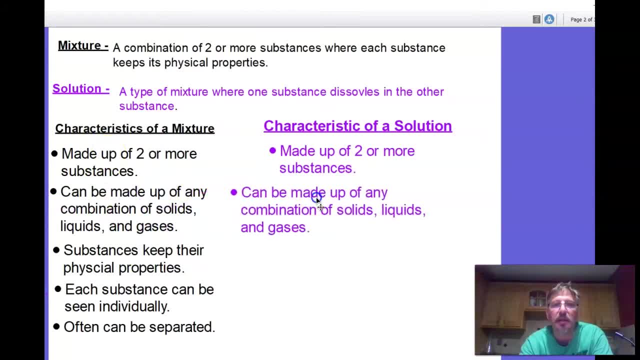 So that's not different. Can be made up of any combination of solids, liquids and gases. Well, that's the same. Now something's missing. Something's a little bit different. One substance dissolves in the other substance, So I bet you have the idea now, which is which? 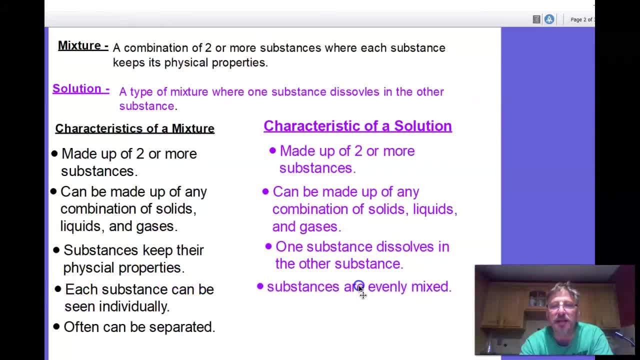 And I like this one a lot. Substances are evenly mixed. You can't see one individual substance anymore, It's just one thing now And the last one- the complete opposite of often- can be separated. This cannot be separated- A few exceptions, but generally cannot be separated. 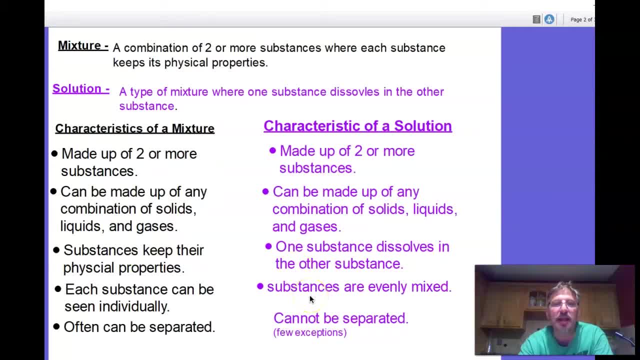 So, right now, finish this list And then go back to your pictures and label the black pepper and water as either a mixture and a solution, And then label your salt and water as either a mixture or a solution. All right, So which is which? 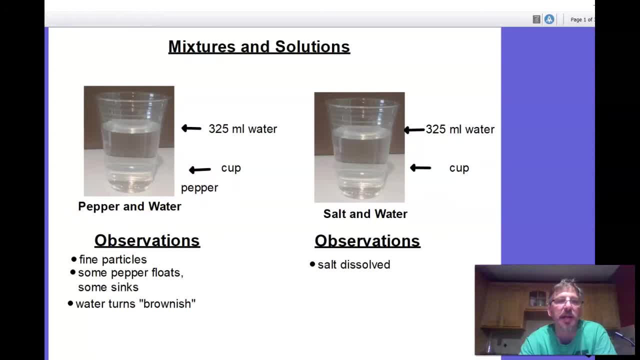 Which one's a mixture and which one's a solution. The black pepper and water. Here It goes. here, Pepper and water is a mixture. You can see each. You can see the black pepper and you can see the water. You can separate it. 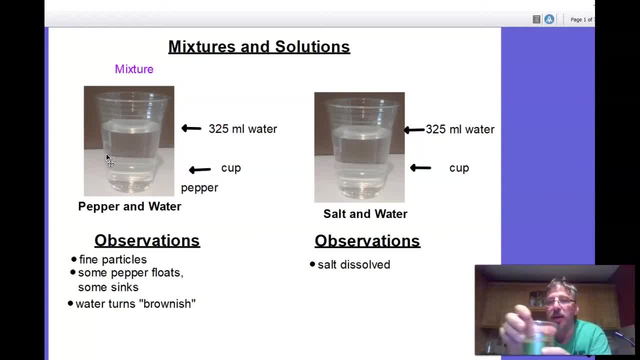 How can I get the black pepper out of the water? Well, I could start pulling out my fingers if I wanted. I could pick up my spoon and I could pull it out So I could see each ingredient. I could see each substance. 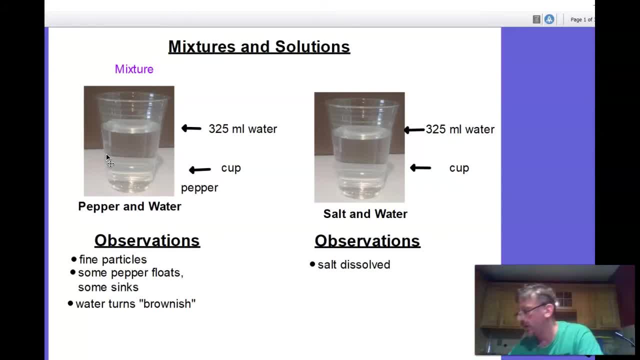 So this one is definitely the mixture. Now, the salt and water is a solution. The salt completely dissolved in the water and I can't see the salt. All I see is clear water. The salt seems to be gone. If you have any salt in yours, by the way, then you should stir it a little more or add more water. 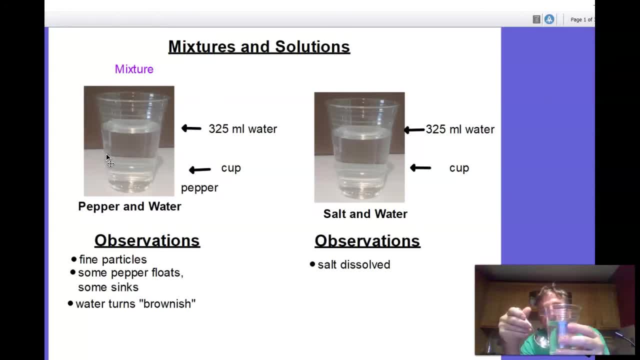 If you put too much salt it gets saturated, But mine is completely void of any salt whatsoever. So this here: the salt dissolved in the water. So it's a solution. I can't take the salt out. I don't see it anymore. 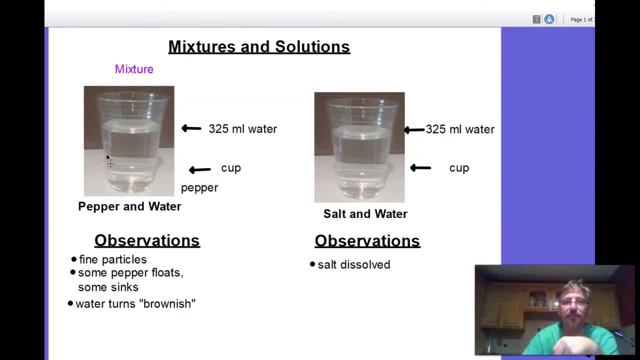 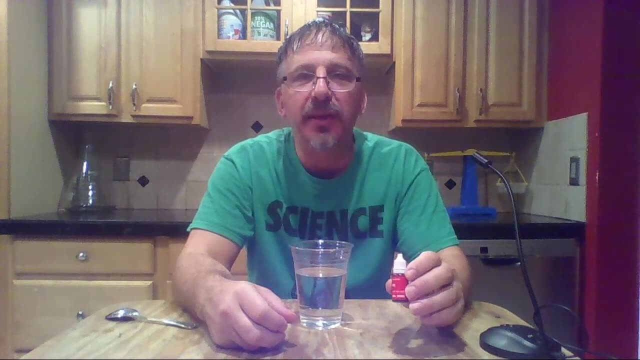 So this one- the salt, cannot be taken out, So go ahead and label this one here as a solution. All right, I have water here and food coloring. I'd like you to make a prediction right now: When I put the food coloring in the water, is it going to create a mixture or a solution and justify your response? 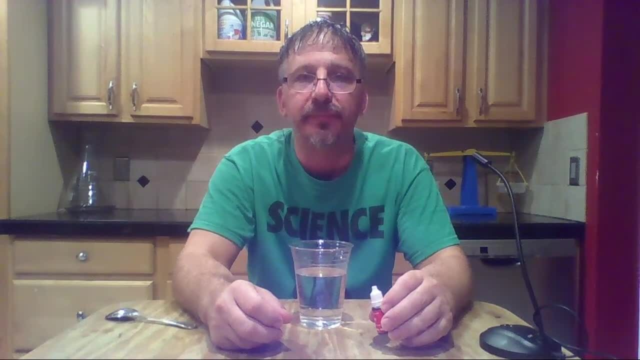 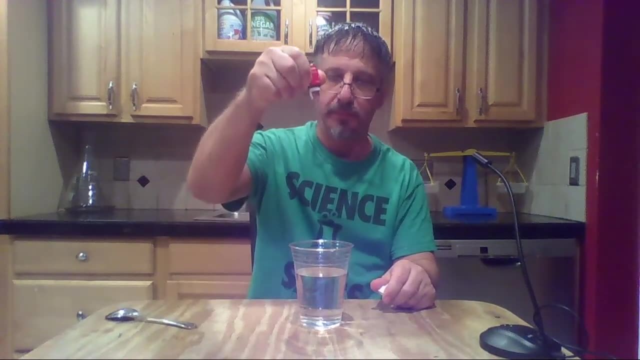 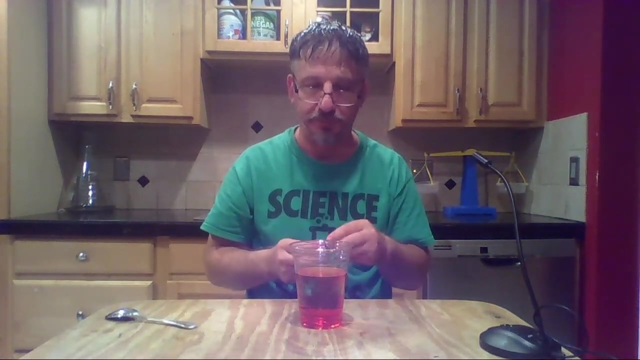 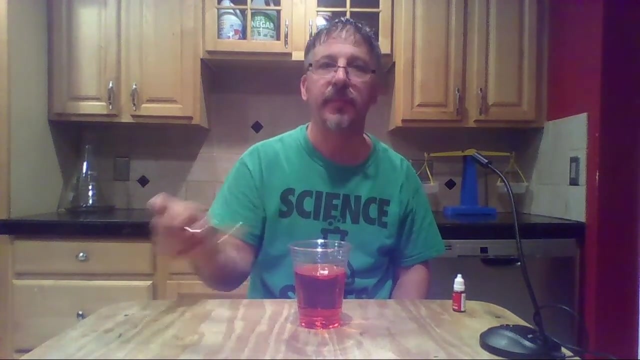 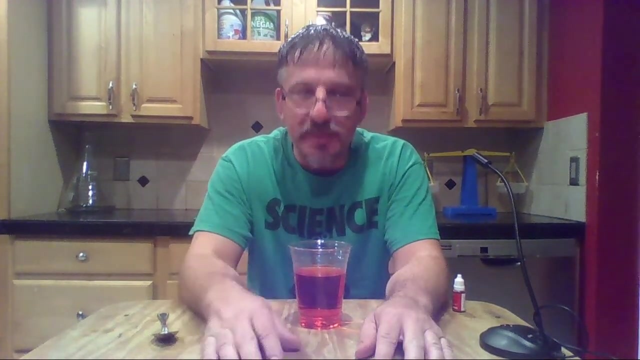 Okay, I'm going to go ahead and put it in, Take my spoon and stir it up. All right, Is that a mixture or a solution? Well, let's go through some of the things. Is it two or more substances? Yeah, 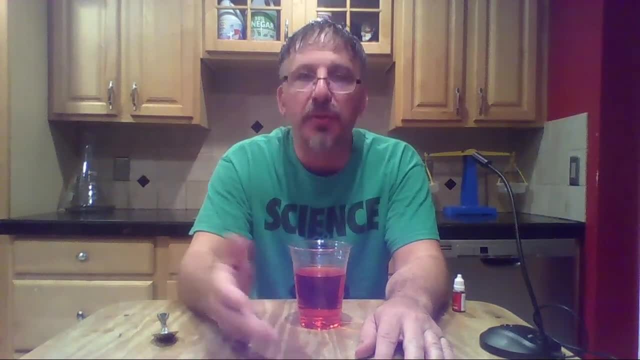 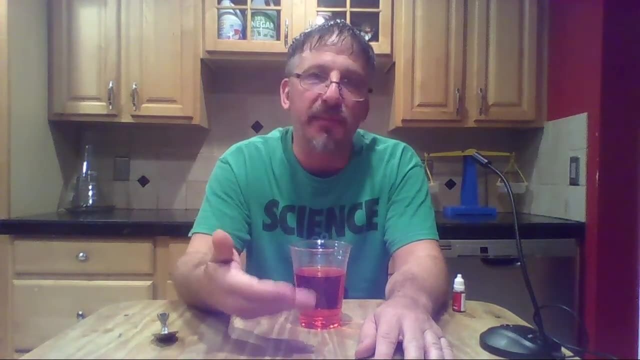 But they both are. Mixtures are two or more substances, And so are solutions. Okay, Is it a mixture of solids, liquids and gases? Well, yeah, It's two liquids: The food coloring is a liquid and the water is a liquid. 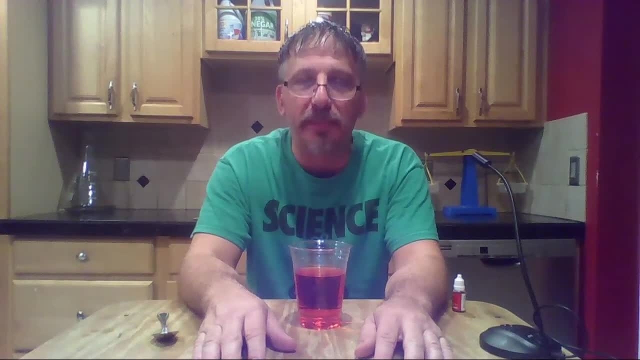 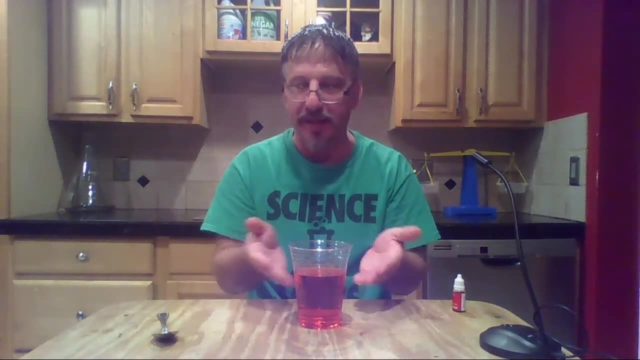 All right. Does each substance keep its own physical properties? No, Actually not, Because now I have red water, I can't get the red out of the water. This cannot be separated, So which one is it? Yeah, It's a solution. 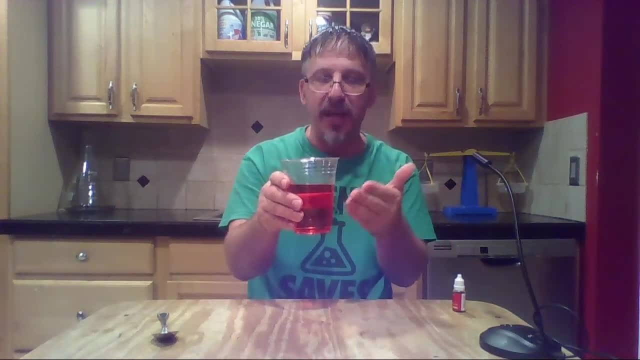 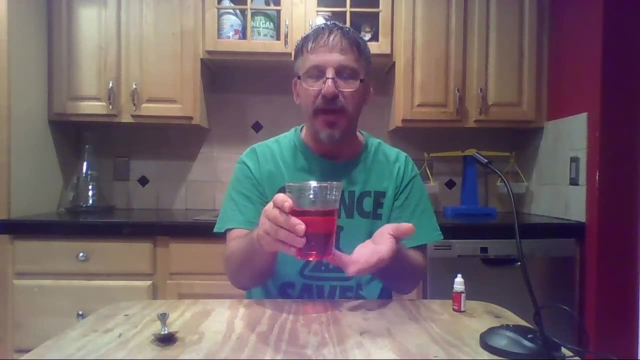 This is evenly mixed. I cannot see where the water starts and the food coloring starts. It's just one thing. It's evenly mixed, It's one substance. So this one here is a special kind of mixture called a solution. All right, 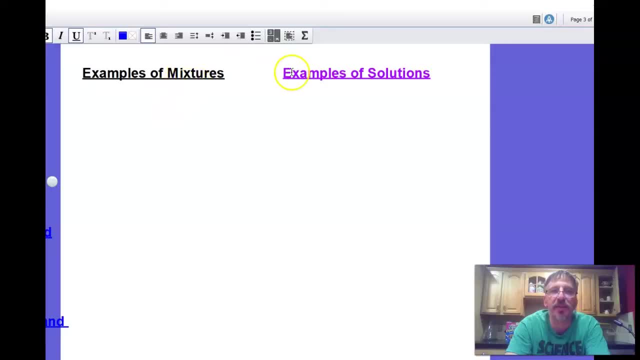 So let's write a list of examples of mixtures and solutions. So skip a line and we're going to make a bulleted list. First, we'll review what we've already done. We said that black pepper and water was a mixture because you could separate it out. 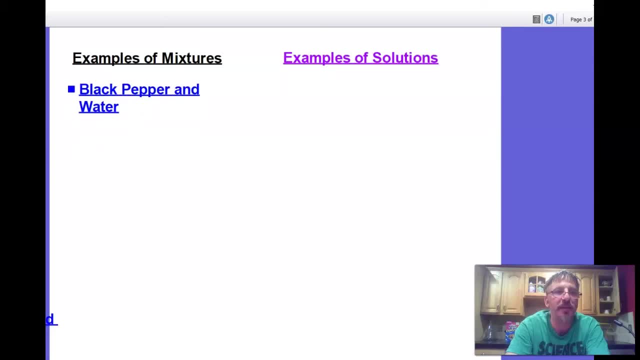 You saw the black pepper and you saw the water. We said salt and water was a solution and the salt dissolved in the water and you could no longer see it. And then we did the food coloring and water and we ended up with red water. 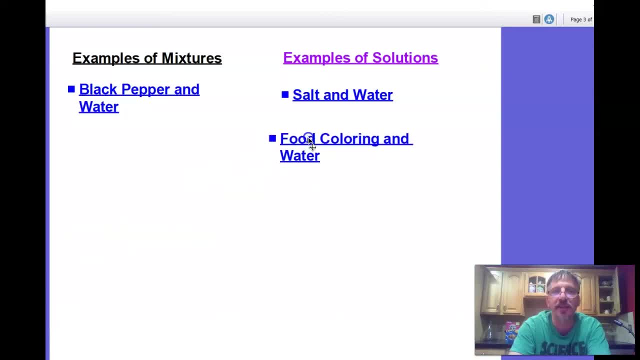 So you can't separate that out and it's evenly mixed. So that is a solution. So I'm going to go over a few more things and you're going to put them in the correct place. I'll show you a few more mixtures and solutions and you put them where they belong. 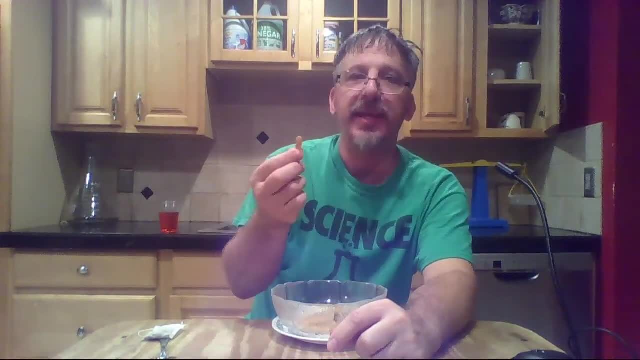 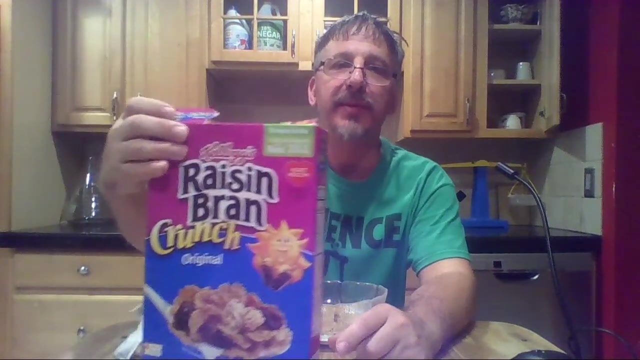 All right. The first one I have here is raisin bran. It has flakes and it has raisins, So is that a mixture or a solution? Put it in the correct place. This is how you spell raisin bran, by the way. 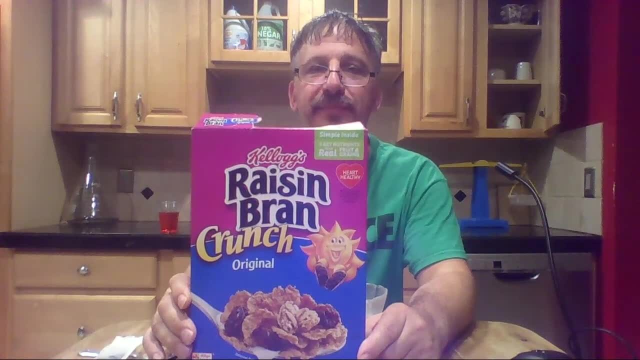 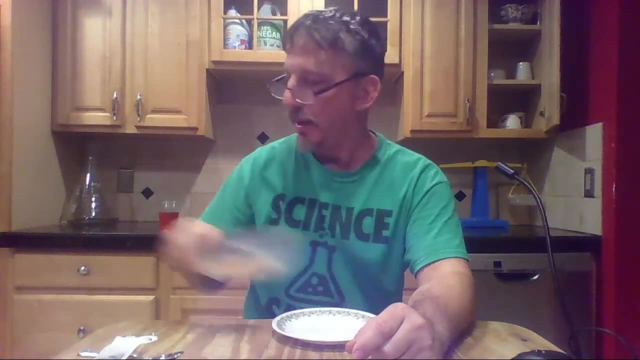 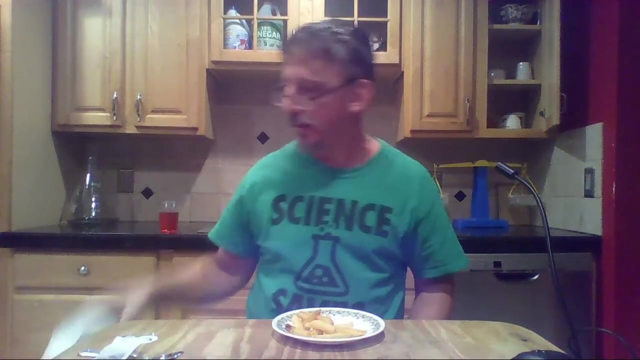 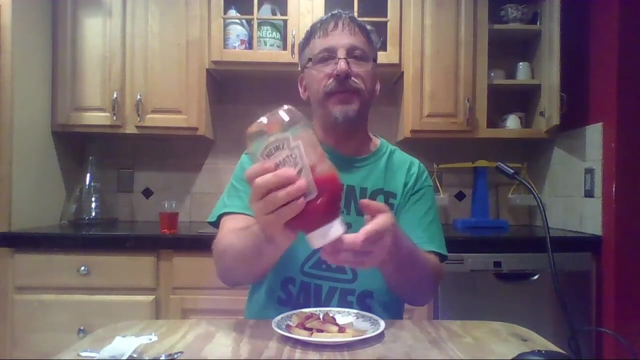 I always have a hard time spelling the word raisin, So I'm going to put it in the correct place. All right, For my second choice here. I love French fries and I love ketchup. Ketchup and French fries Mixture or solution. 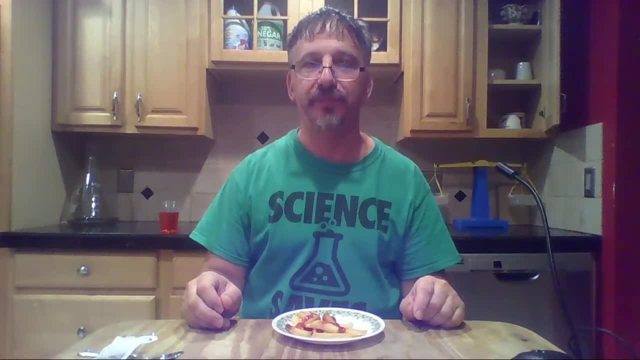 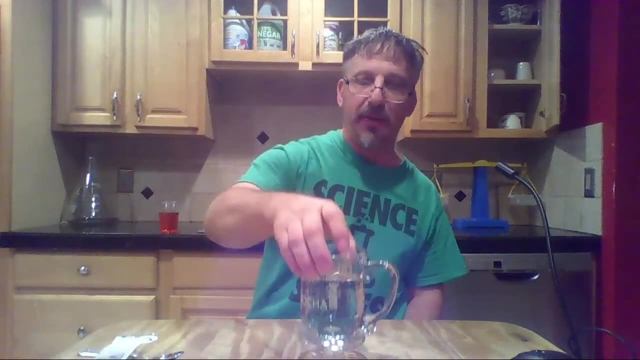 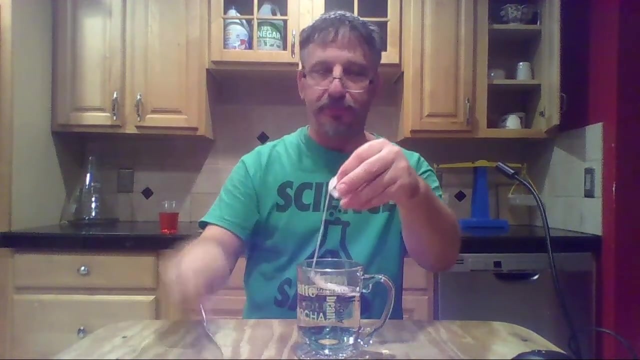 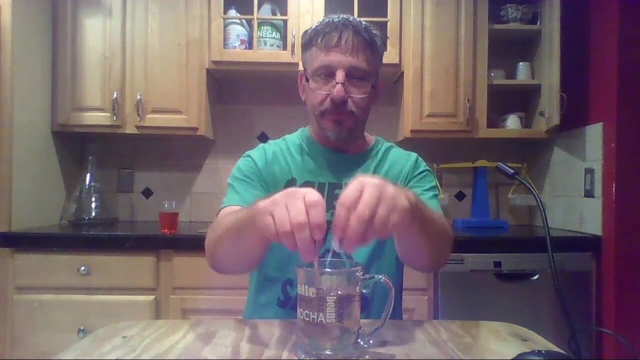 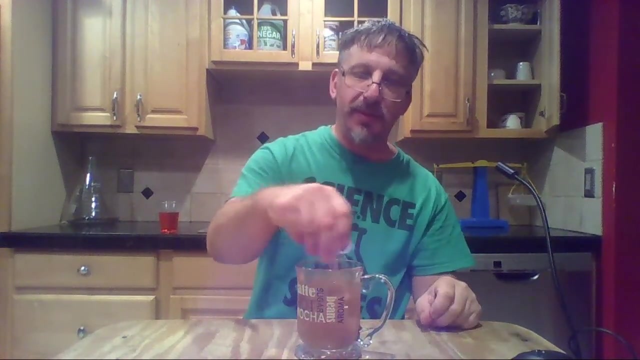 Put it in the correct location. And lastly, I have some hot water here And I have a teabag. Put it in, Dip my teabag in, And now my water is turning nice and brown, All right Now. stirring accelerates the dissolving process. 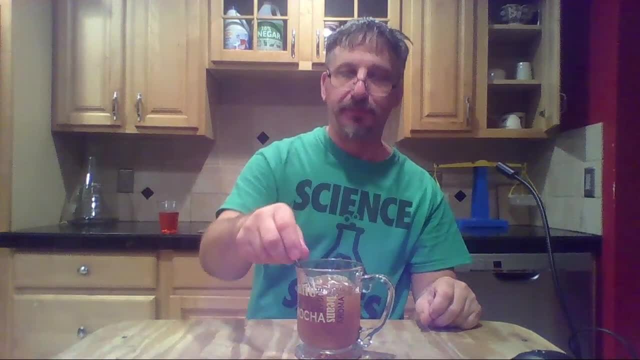 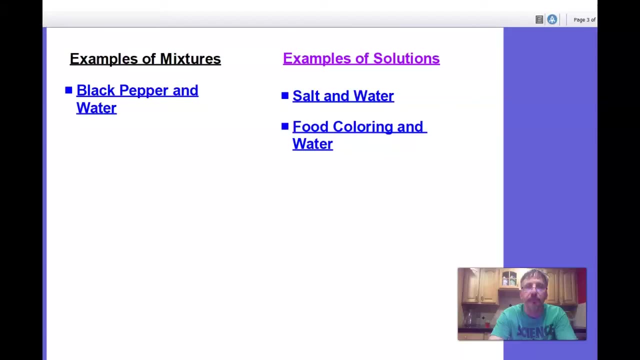 Oh, did I give it away? All right, So hot tea or iced tea? would that be a mixture or a solution? All right, So first thing we looked at was raisin bran. We were able to pull the raisins out of the cereal. 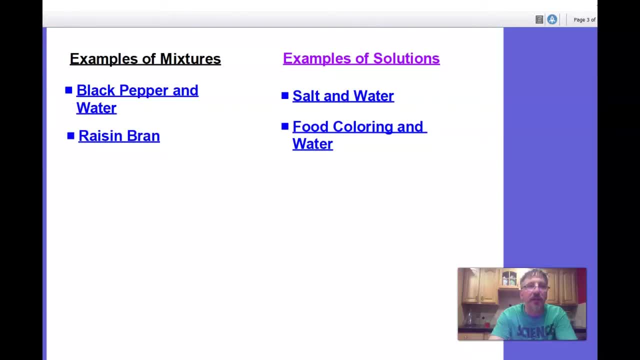 So that is a mixture: Ketchup and French fries. We saw the ketchup laying on top of the French fries. So that is also a mixture. And then we saw inside the hot tea or iced tea is the same. The water turned brown and then it became uniform and evenly mixed. 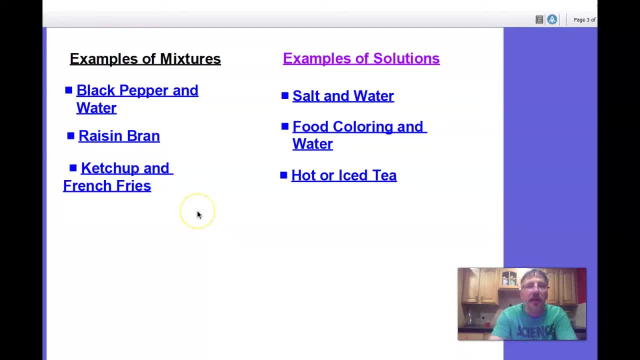 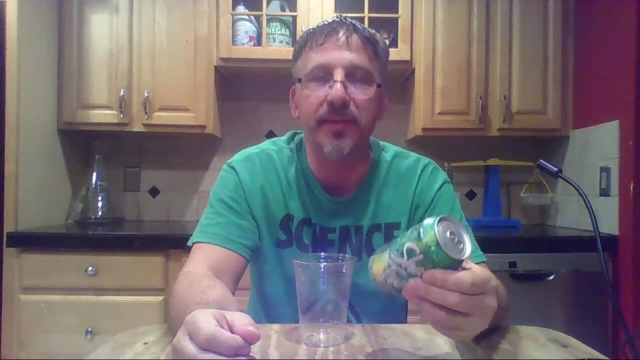 That is an example of a solution. Please add two more examples of mixtures and two more examples of solutions to your notes. I would like to use soda as a good example, because it is a mixture of solid liquid and a gas. It has sugar in it. 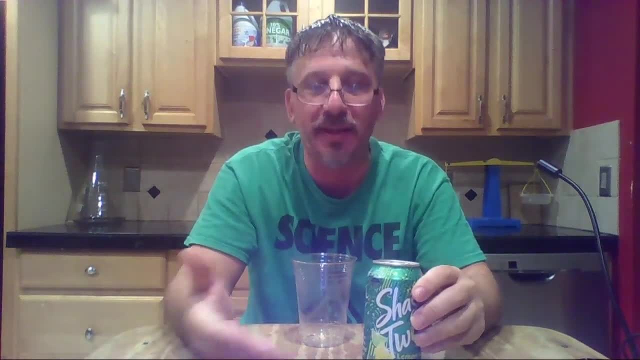 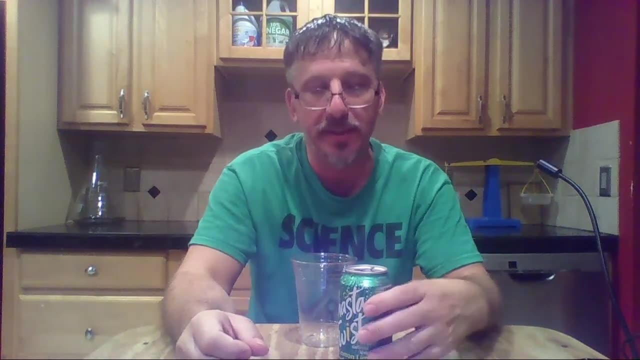 That is a solid. It has corn syrup in it. That is a liquid- Many other ingredients, But it also has a gas called carbon dioxide in it And that is what makes that noise. So this is a mixture of a solid, a liquid and a gas. 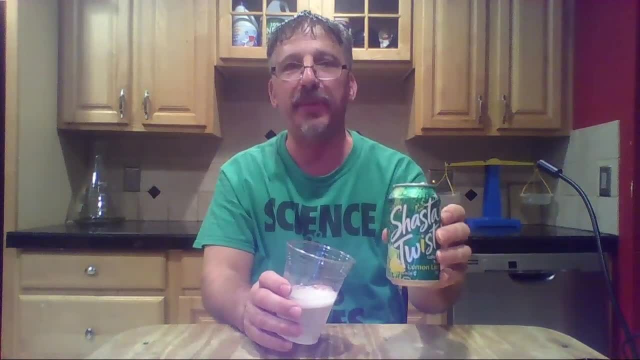 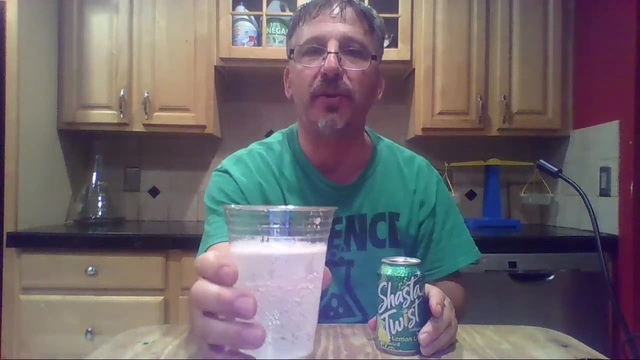 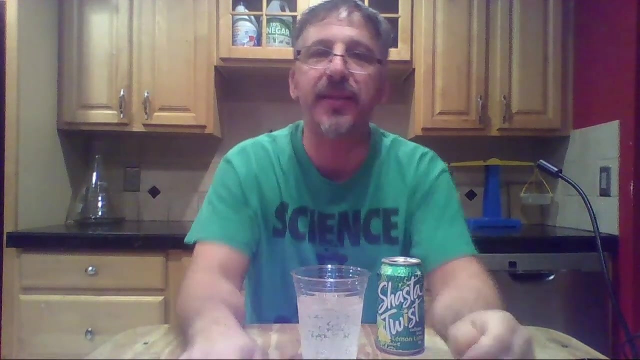 This stuff is called shasta milk. It is a twist. It is probably a generic Sprite-type soda, But anyway, all that stuff that is making the fizz up here, that is all caused by carbon dioxide, which is a gas, So add that to your list of solutions. 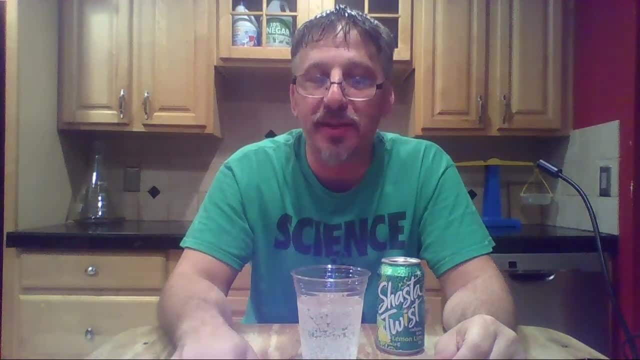 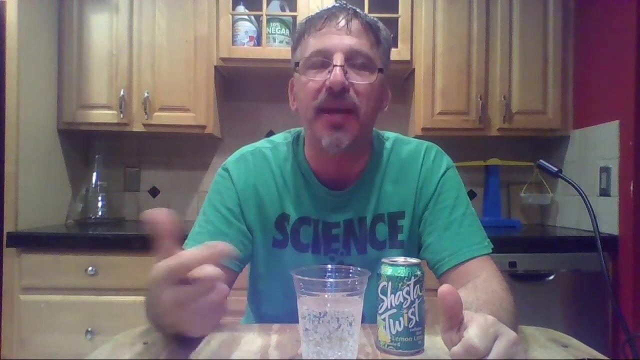 One other gas you might want to consider is the air that you breathe. The air that you breathe is 78% nitrogen, 21% oxygen and 1% carbon dioxide, So it is a mixture of many different gases. So we have talked about many different solids, many different liquids and many different gases. 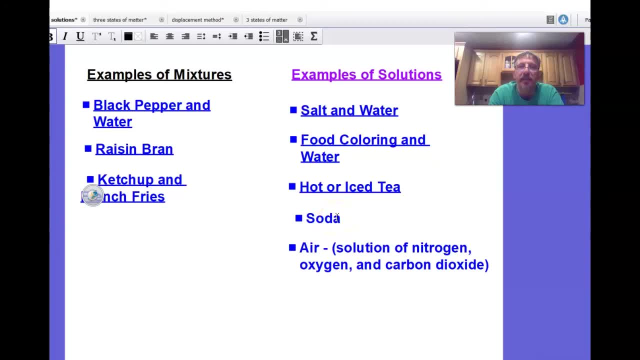 Alright, so here is an updated list of the examples of solutions and mixtures. We added soda. Remember, soda is a solution made up of solids, sugar, liquids, water and gas carbon dioxide. And we talked about air and how air is a solution of nitrogen oxygen and carbon dioxide.